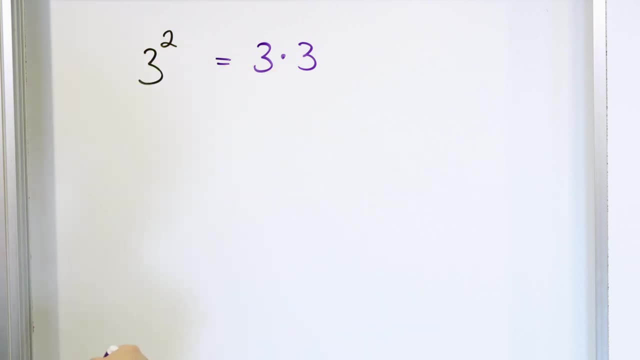 many 3s do I have here? I have 2 of them, because it's 3 squared. So that's why I say it's a shortcut for multiplication. What you do is you take the base, the bottom number, and you multiply it by itself. And how many of these are here in the multiplication It is. 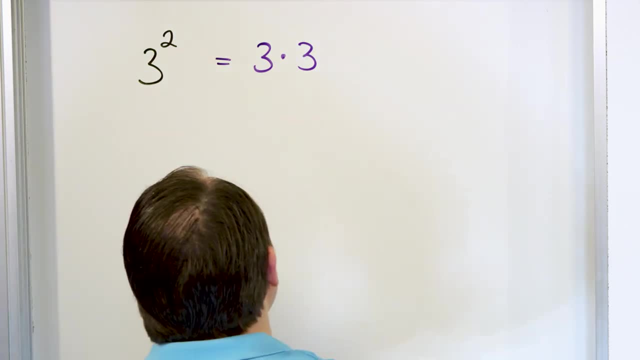 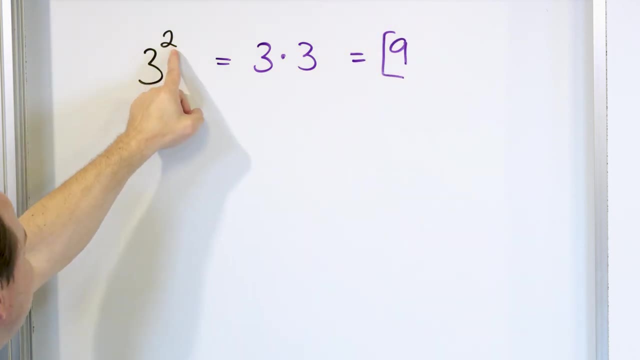 the number that we have in the exponent. All right, So what is 3 times 3 anyway? 3 times 3, as you know, It is 9.. So we can say that 3 to the power of 2 is 9.. We can also call it 3 to the exponent. 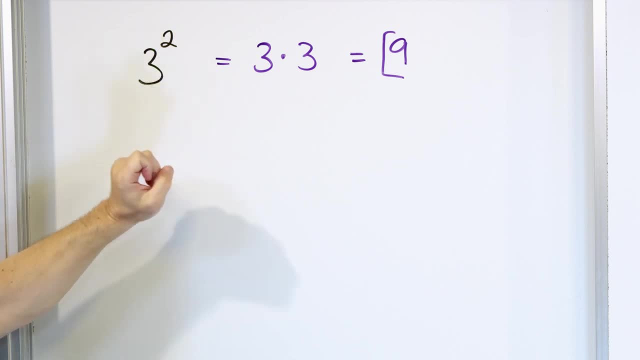 of 2 is 9.. And we can also call it, because 2 is a special exponent. we say 3 squared is 9.. Now you might say: why do I care about that? That doesn't seem so helpful, You're. 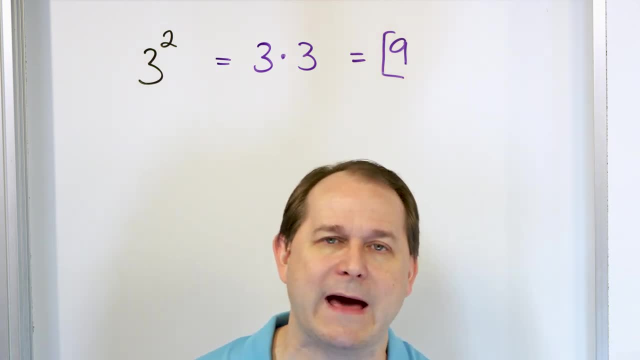 just going to have to trust me a little bit that when we get a little farther in math, exponents pop up all over the place in our equations. One simple example: when you get a little farther along and calculate how much gravity is between two objects like the Earth and the moon, there's going to be a. 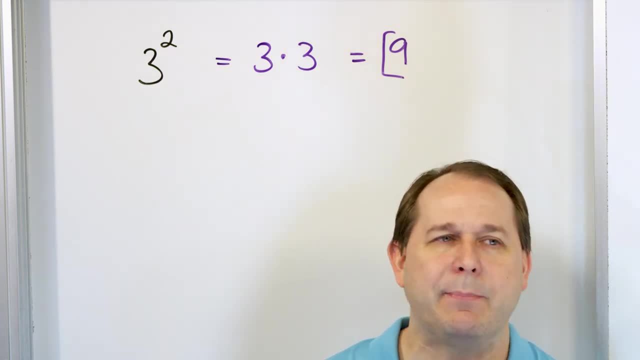 square an exponent of 2, in that calculation It pops up in nature all the time. So let's get some more practice here and take a look at some additional examples. What about 2 to the power of 2, or 2 to the exponent of 2?? We can also call it 2 squared. How would 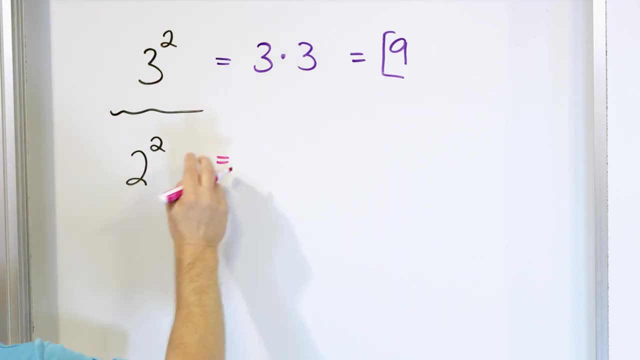 we write that down, All right. Well, what we do is we take the bottom number and we multiply it by itself. So it's this many times times itself: We have 2 squared, So we have 2 of them, because the exponent is a 2.. 2 times 2 is 4.. So we say 2 squared is 4, or 2 to. 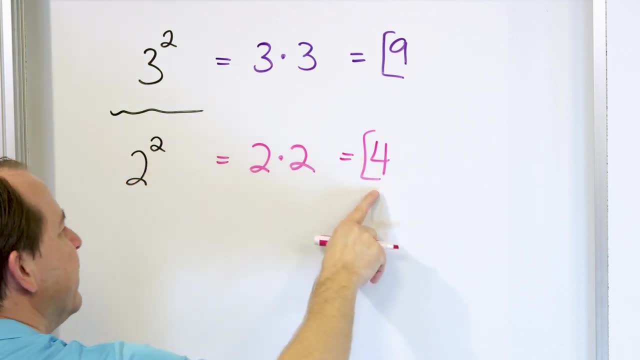 the power of 2 is 4, or 2 to the exponent of 2 is 4.. All of those mean exactly the same thing. All right, Let's take a look at another power of 2, 5 to the power of 2.. How would 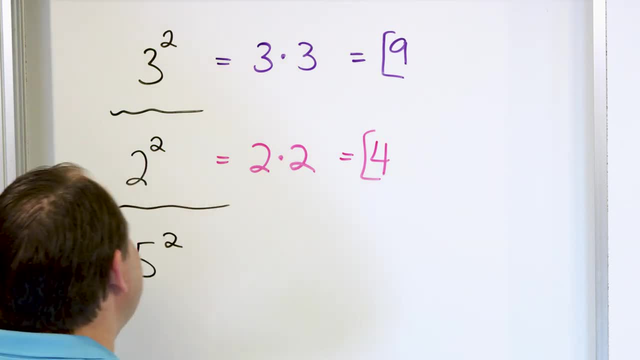 we write that down. We're always, always multiplying by ourself, by itself. So it's 5 multiplied by itself. 5 times 5 is 25.. So we say that 5 to the power of 2 is 25.. All right, Now let's change the. 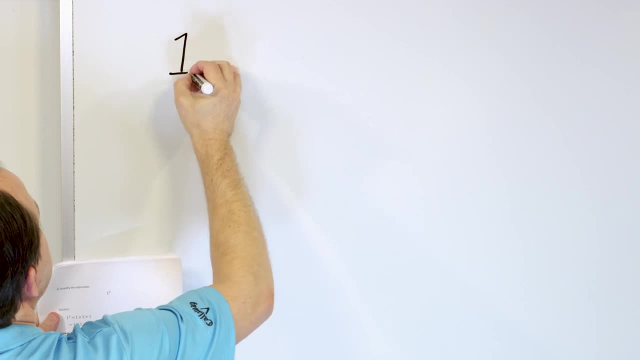 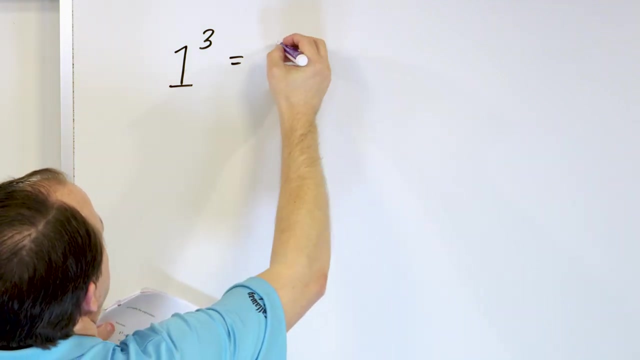 exponent a little bit and mix it up a little bit. Let's say we have 1 to the power of 3.. Now what do you think you do here? The exponent is telling you how many times you multiply by itself. So 1 times 1, that would be 1 to the power of 2.. But we have 1 to the power. 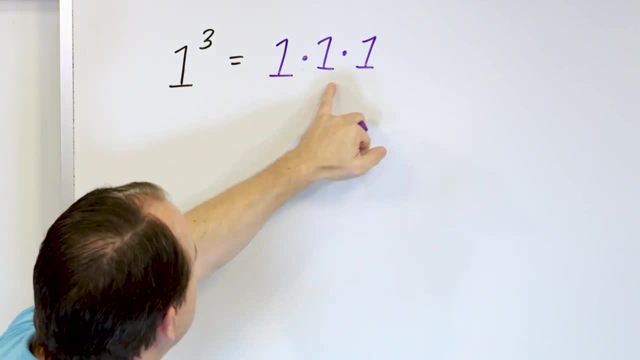 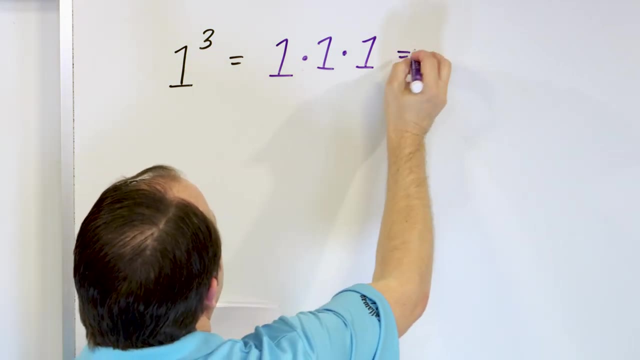 of 3.. So it has to be times itself again. You see, the number of times I have on the board here, multiplied by itself, is the same as the exponent. That's what the exponent is Now, since you have multiplication, remember. 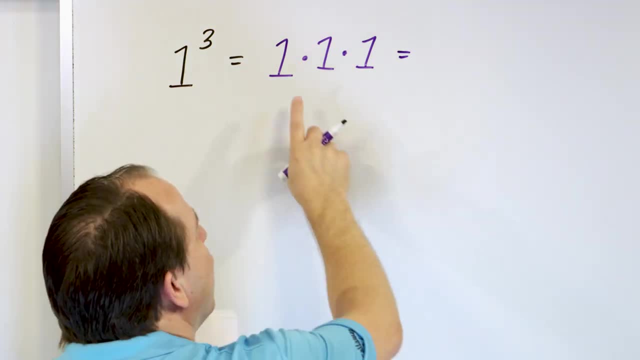 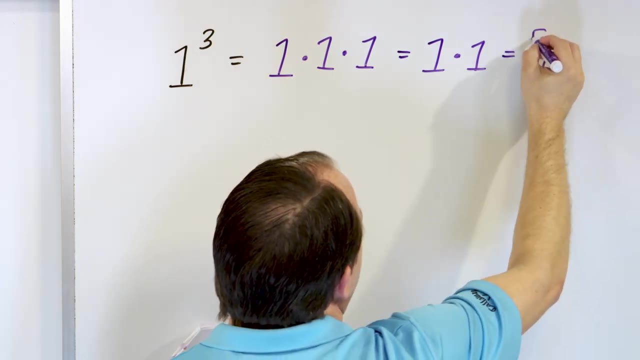 order of operations means you go left to right. multiply 1 times 1 is 1.. And we still have to multiply by this 1.. So we're multiplying again And 1 times 1 again is 1.. So all I've 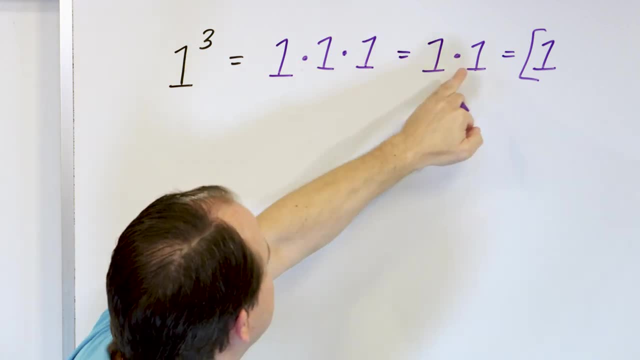 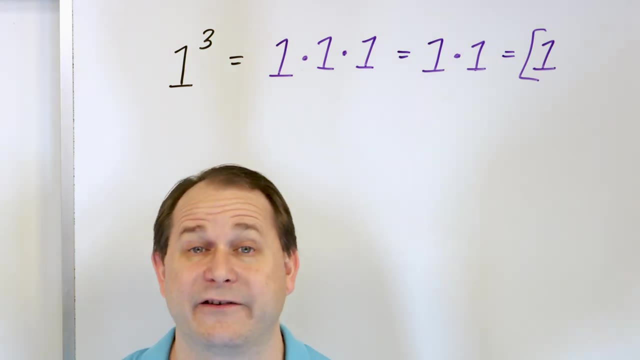 done here is: I multiplied the first 2 to give me 1.. And I still have to multiply by 1 again And I get 1.. Now, 1 is a special number. It doesn't matter what exponent you raise it to The answer. 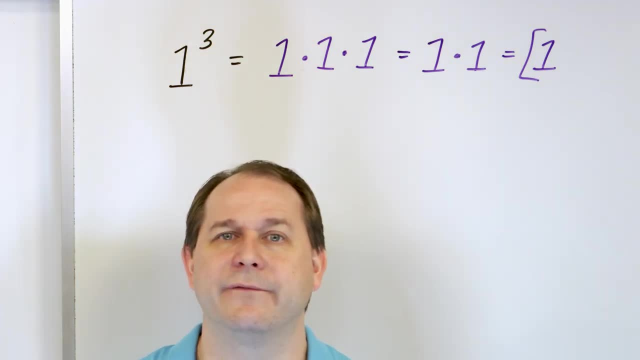 is always what 1.. 1 to the power of 4 is 1 times 1 times. 1 times 1 equals 1.. What is 1 to the power of 19?? Still 1.. What is 1 to the power of 100?? 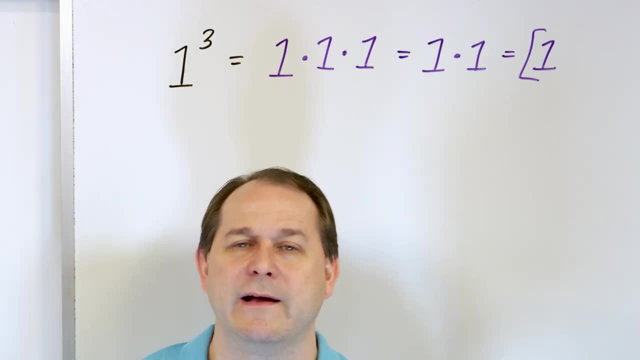 Still 1.. What is 1 to the power of 2,034?? Still 1, because all you're doing is multiplying times 1, over and over again. All right, What about 8 to the power of 4? 8 to the power of 4.. 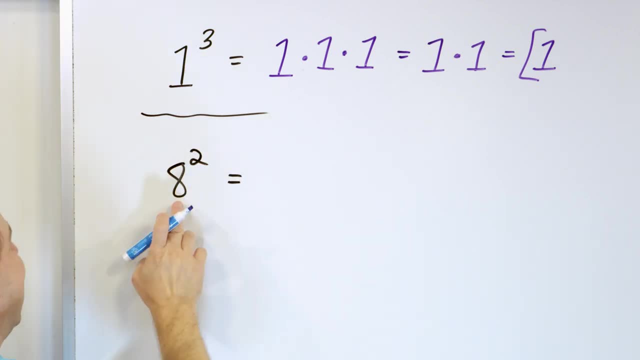 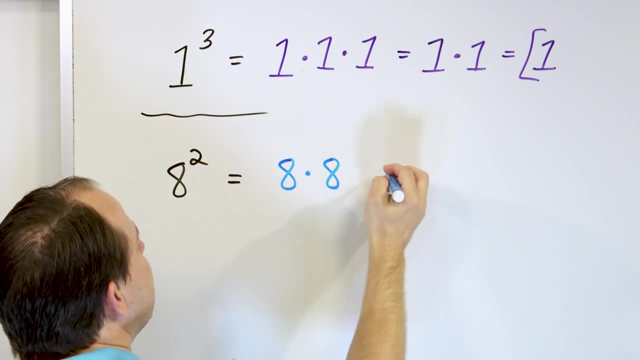 1 to the power of 2,034 is 1.. power of 2.. 8 to the power of 2.. Well, we take the bottom number, the base, and we multiply it by itself. We have to have 2 on the board, because we have a power of 2.. 8 times 8 is what? 64.. 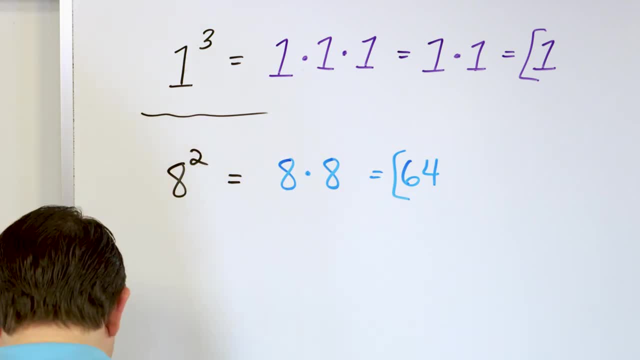 So we can say that 8 squared is 64, or 8 to the power of 2 is 64.. All right, let's move right along here. What about 10 to the power of 2? 10 to the power of 2.. Same thing, Bottom number is. 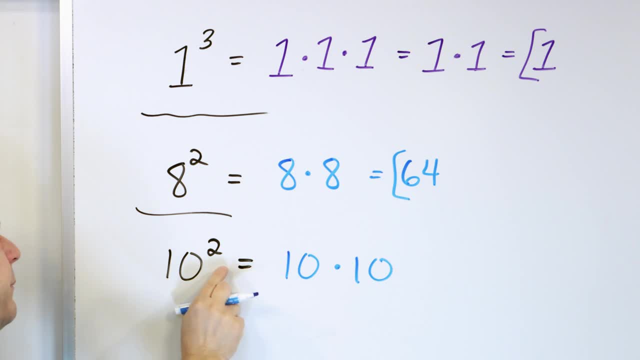 the base, We multiply it by itself and we have 2 of them here, because the exponent is 2.. 10 times 10, you know from your multiplication tables- is 100. So the answer is 100.. And you might say: 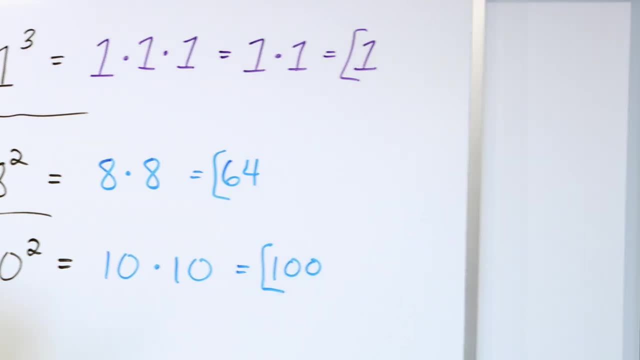 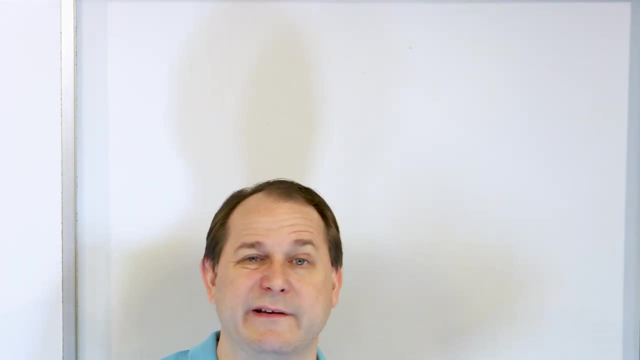 why is he doing power of 2 so many times? And the truth is, as I mentioned before, the power of 2 pops up so much in real life. It pops up in gravity, It pops up in electricity and magnetism. It pops up. I could go on and on. The power of 2 is just special. somehow It pops up everywhere. 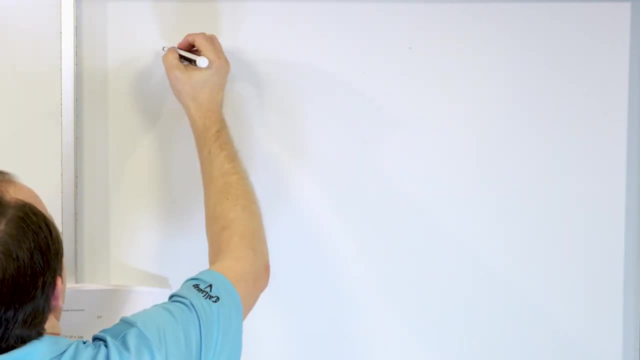 So we do that one a little more. Now for our next one. what about 3 to the power of 3,? right, So 3 to the power of 3.. What does this actually mean? It means you take the bottom number 3, and you multiply it by itself And we: 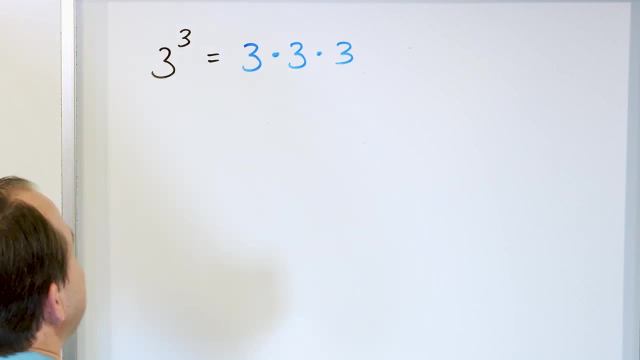 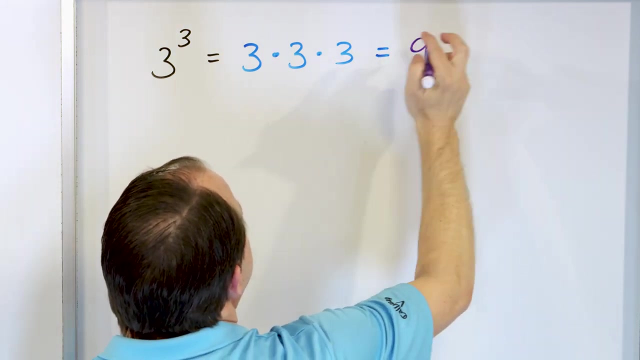 have to do that three times here because the power is 3, right. So when we get the answer, we multiply left to right. 3 times 3 is 9.. But I still have to multiply by this final 3.. What is? 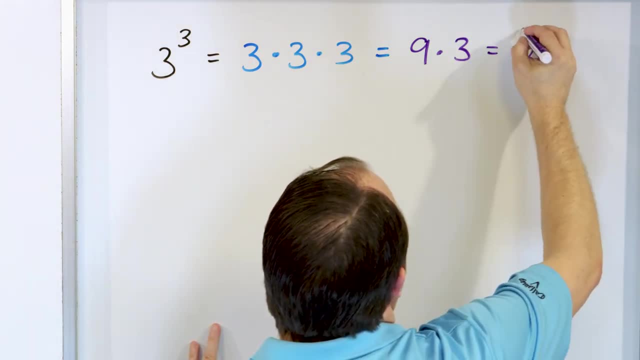 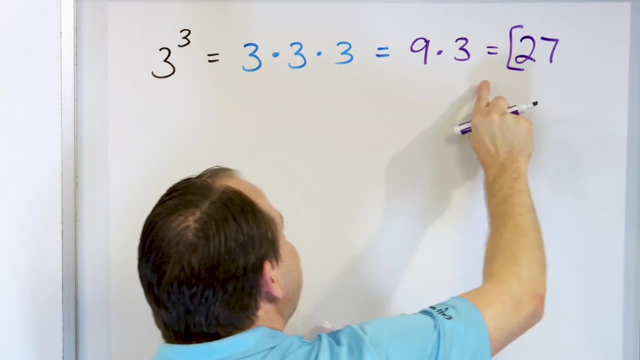 this 9 times 3?? That's 27.. And so the answer to 3, to the power of 3, is equal to 27.. So we have 27.. These two things are interchangeable Anytime you see this. it just means this And it's a. 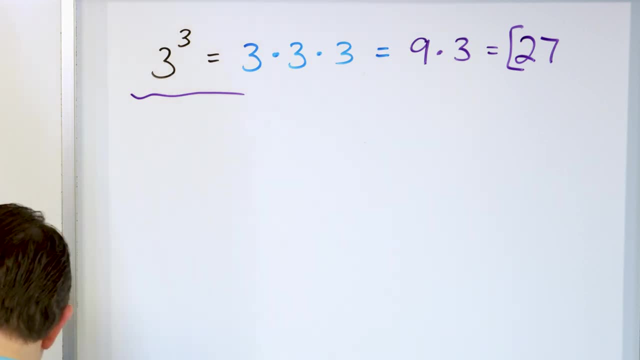 shortcut way of writing out all of this multiplication. All right, Let's take a look at- We're almost done. actually Take a look at 4 to the power of 2.. What does 4 to the power of 2 actually mean? It means we take the base 4, and we multiply it by itself. And what is 4 times 4?? 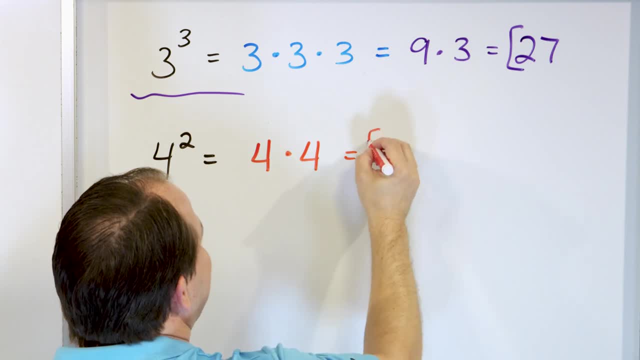 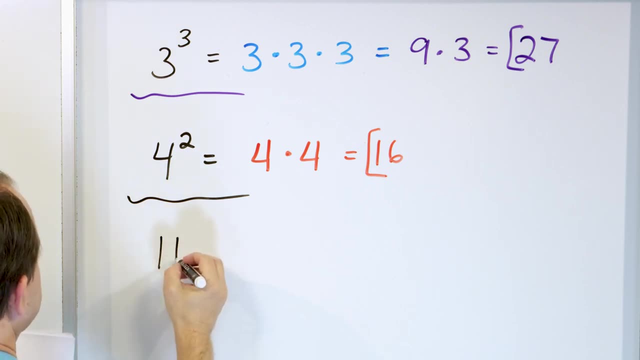 We have two of them here, because of the power of 2.. 4 times 4 is 16.. So the answer to that problem is 16.. You see, once you get the hang of exponents, they're actually quite easy. What about 11 to? 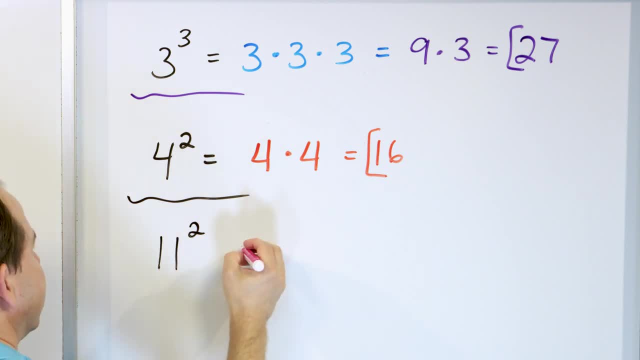 the power of 2?. 11 to the power of 2 means that we take the 11, and we multiply it by itself. We have two of them here because we're squaring it Now. you might remember this or you might not. 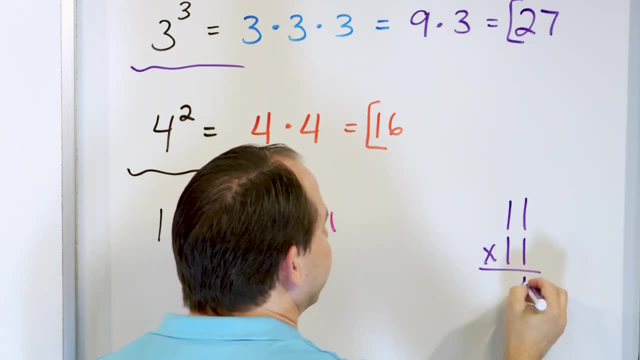 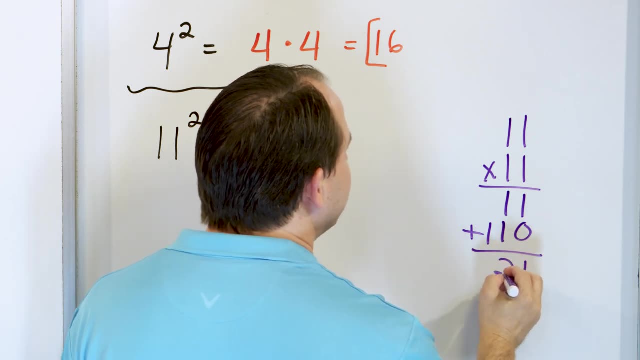 If you don't just go over here and multiply. We have to multiply these. 1 times 1 is 1.. 1 times 1 is 1.. Drop 0.. 1 times 1 is 1.. 1 times 1 is 1.. Add: We have a 1, a 2, and a 1.. You might. 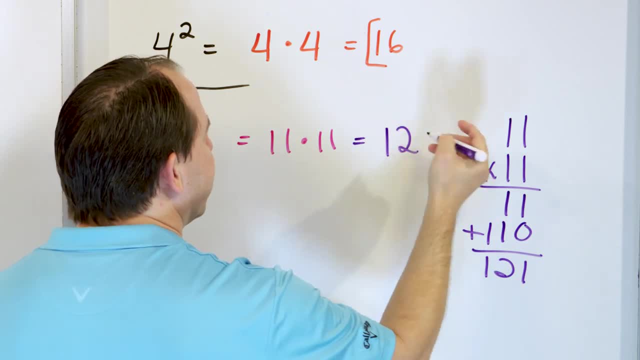 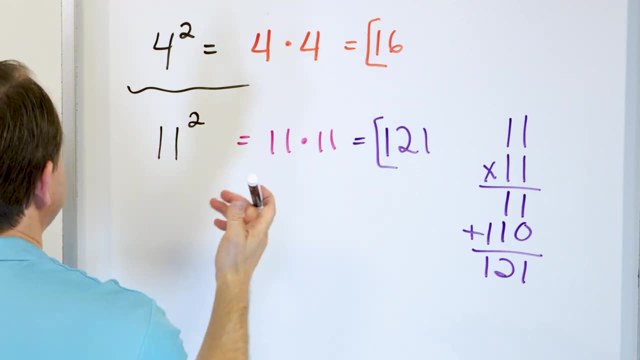 remember that 11 times 11 is 121. But if you don't just write down and multiply there, The answer is 121.. All right, now here's our very last problem. Let's take a look at 2 to the power of 3..